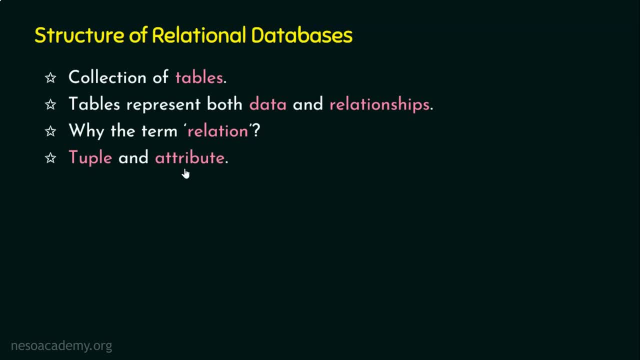 And in relation, rows are referred as tuple and columns are referred as attributes. And when we talk about the relational database, we saw about the relation instance. What is a relation instance? Instance means it is the data that is actually at a given instant of time. When we talk about 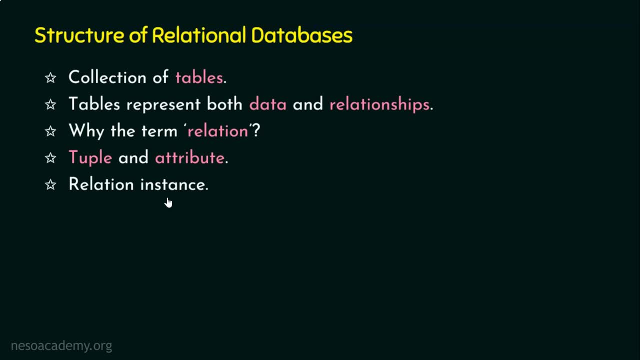 relation instance. it is actually the snapshot of the table or the relation and the data present at a given point of time which is actually referred as relation instance. Please be noted that relation instance is different. database instance is different. Anyway, in this presentation, 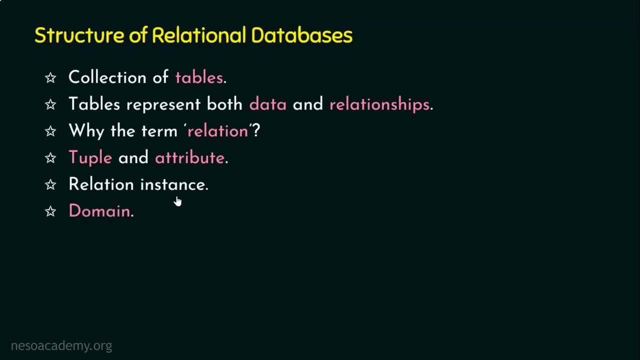 we are going to clarify that And we also have seen about the domains and we also have seen when a domain is atomic. and we have seen about null values, sorted and unsorted relations in the previous presentation. In this presentation, let's focus on the database schema First. 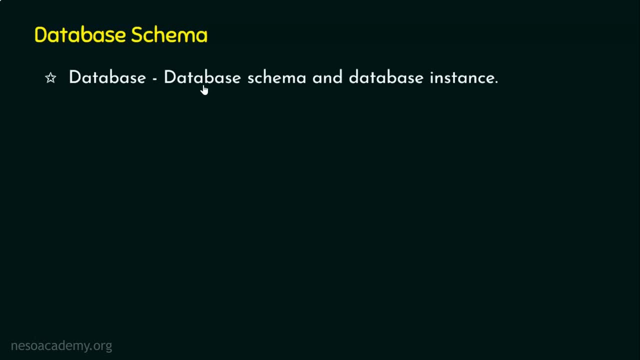 we should understand is in a database. we are going to focus on the database schema and database instance. Remember, when we have a collection of tables, all collection of tables are in a single database And when we talk about the database schema, this is actually the logical design of the database Before we go and execute the physical 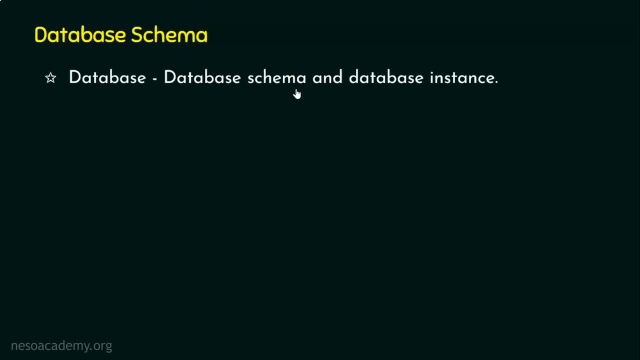 aspects. we logically create the database design at the higher level right. So this is actually the logical design of the database. The logical design of the database is actually referred as the database schema And talking about database instance, this is actually the snapshot of the 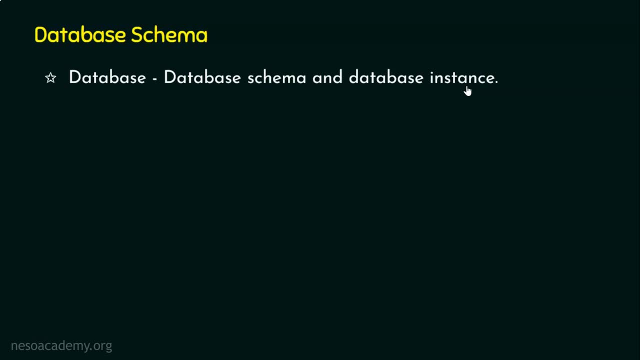 database. It means this is the database. This database may contain n number of relations. All the data present in all the relations collectively at a given instant of time is called as the database instance And normally databases keep updating because relations or tables keep updating And that's why databases are also keep. 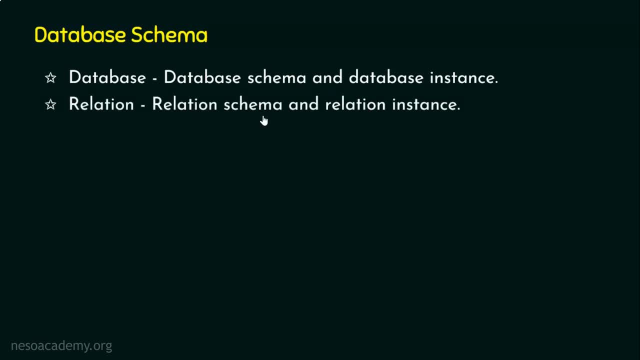 updating. And when we talk about the relation, the relation schema and relation instance- we have already seen about this in the previous presentation. The relation schema is like the type variable, Say, for example. if we are declaring a variable x of integer type, it means x is of. 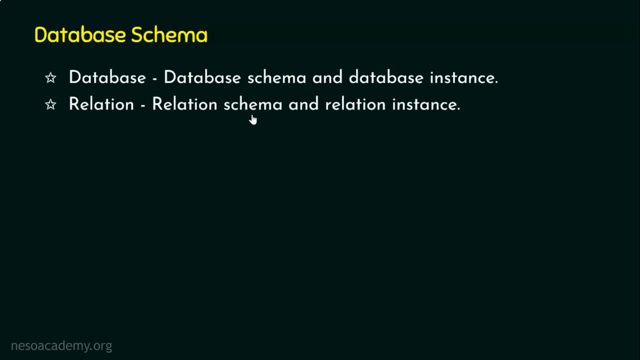 integer type. So this relation schema is like the type definition in the programming language. This is fixed, But the value that x is storing it keeps changing. So that is actually relation instance. So relation instance is like the value of a variable which changes with time When we 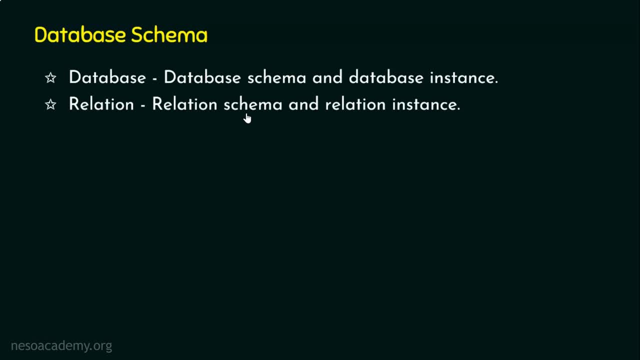 talk about the relation schema. this is the logical structure of the relation. What a relation will contain All attributes? What a database contains All tables. So this contains collection of tables and its relationship, And this contains collection of attributes. 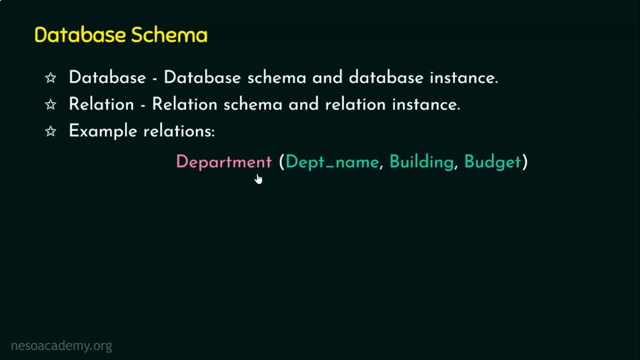 I will show you two example relations: Number 1, the department relation and number 2, the instructor relation. When we talk about the schema, this department and instructor, all are relations. But what is a database Collection of relations is the database. So 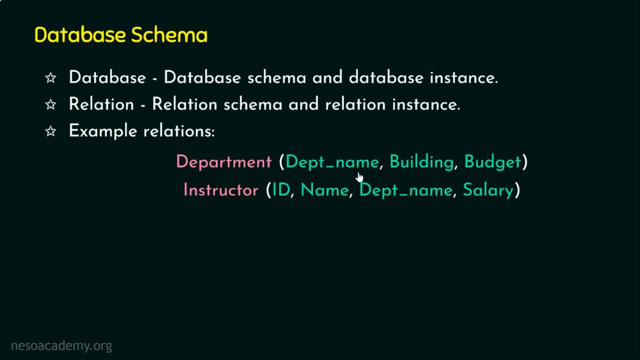 when we talk about the department relation, just see the department name. the building and the budget actually are the three attributes under department relation. Talking about the instructor relation, the instructor ID, the name of the instructor, the department name and salary are the attributes in 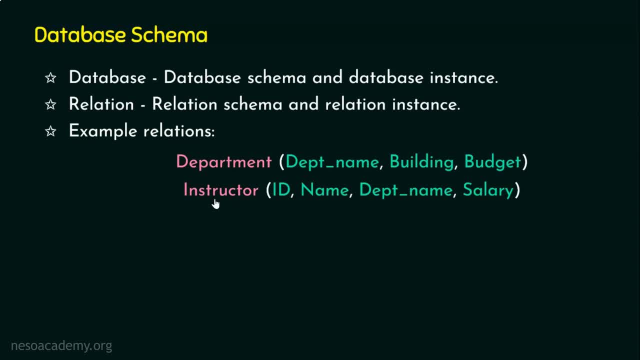 the instructor relation. Every instructor will be belonging to a department and that's why there is a common attribute here: the department name in the department relation and the department name in the instructor relation, And this is how the relationship among tables or relations are actually established. The examples that we are seeing without any data, the relation schema I am. 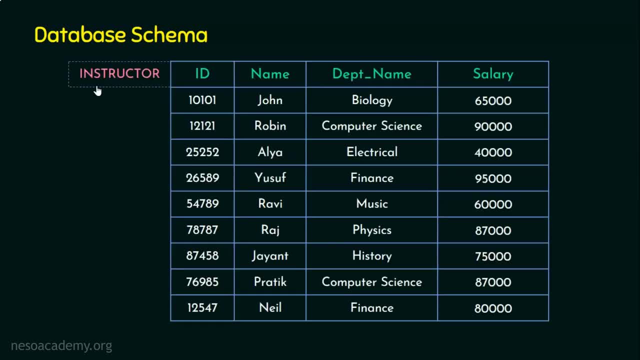 just presenting. Let's take the instructor relation. now, This instructor relation. when it contains the data, it looks like this: All these are tuples and these are all attributes. ID name, department name and salary are attribute. At this time, we have nine rows with these values, but we can't. 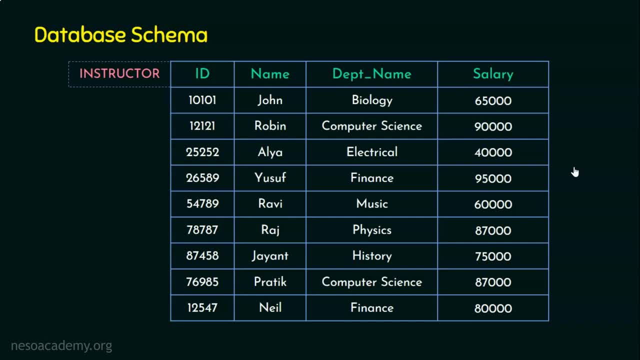 guarantee that this relation will be forever like this, because databases keep changing, The relationship between the two is not the same. The relationship between the two is not the same. Maybe the salary might be increased, the instructor might have quit the university, or a new instructor. 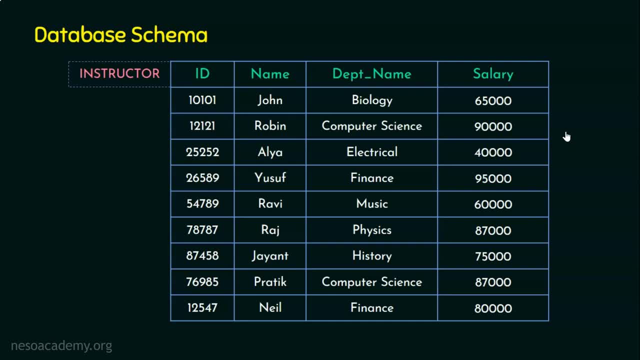 might have joined. So relation keeps changing. The data present in a relation at a given time is the relation instance and here is the relation schema. I'll show you one more example, not the department example, what we have seen in the previous slide. I will show you something different. 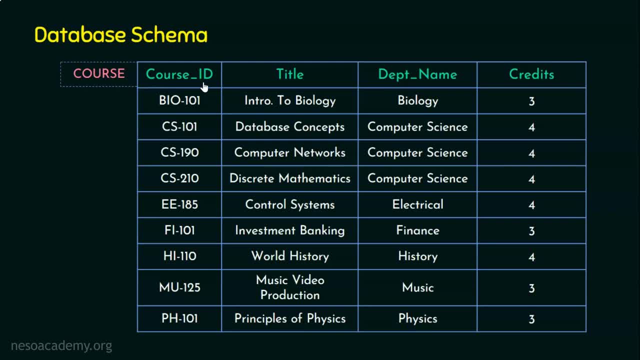 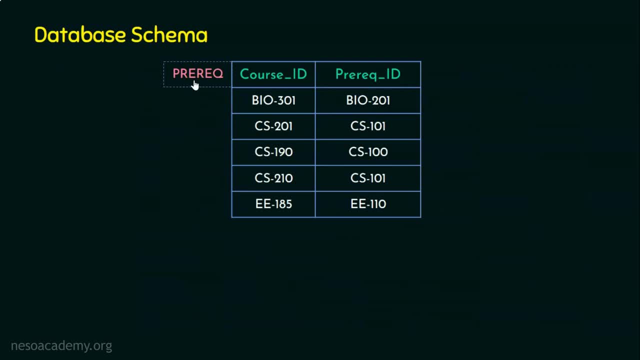 here, which is the course relation, And this course relation contains course ID, title, department name and credits. Let's see One more example: the prerequisite table. This prerequisite table shows the course ID and what's the prerequisite ID for that course. Say, for example, if you want to undergo bio 301 course. 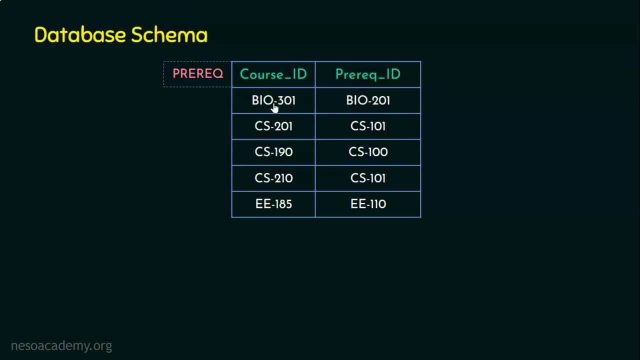 then you should have already completed bio 201 course. So this is how the relation schema are actually organized. But what's the title of this presentation? Database schema, isn't it? But we are focusing on relation schema. Actually, a database is a collection of relations. I'll. 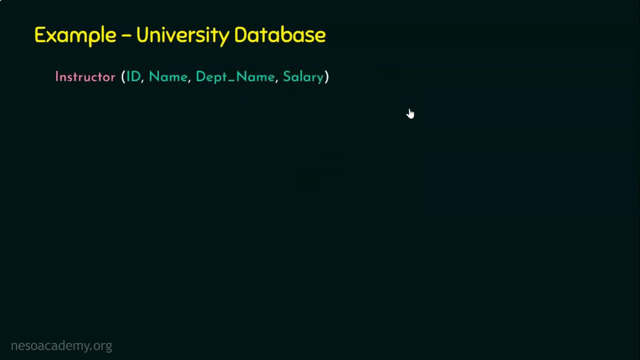 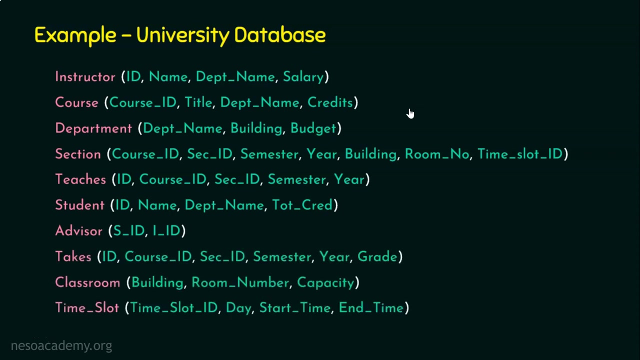 show you an university database where we see multiple relations: the instructor relation, the course relation, the department relation, the section relation, the teachers relation, the student relation, the advisor relation, the takes relation, the classroom relation and the time slot And all the instructor related data are stored in the instructor relation. 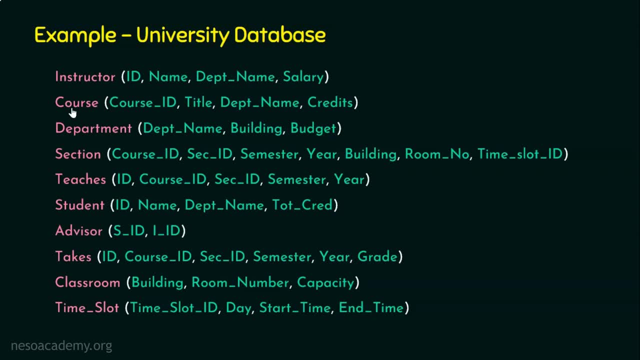 which contains ID name, department name and salary. The course related information in the course relation, department related information in the department relation and section related information in the section relation. Now talking about the next relation, the teachers. this is actually the relationship. a teacher teaches. 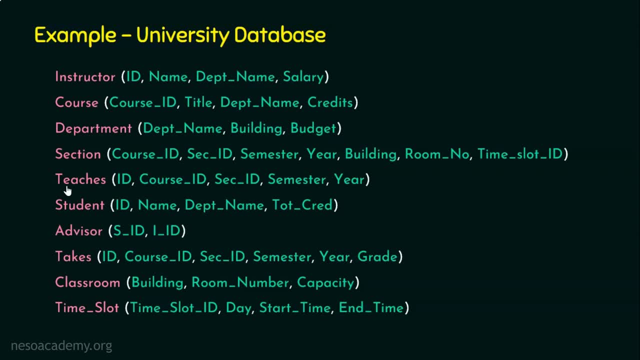 an instructor teaches to whom students, So this teaches is a relation that is actually maintaining the relationship between the teacher and the student: The teacher ID and what course he has taught and for what section he has taught and which semester and which year and what about. 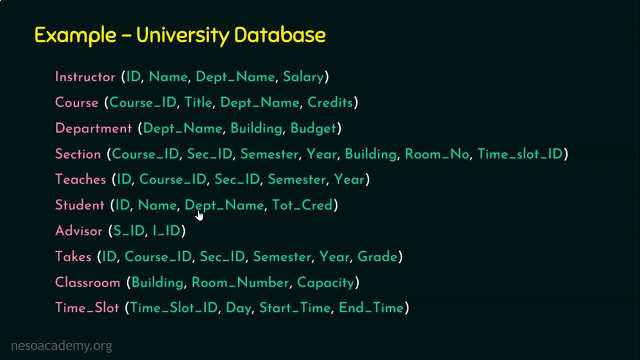 student relation. The student relation contains student ID name, department name and total credits earned In coming to the advisor relation student, if they want any advice or if the teacher or instructor wants to see the progress of the student, then we need to know which student is belonging to. 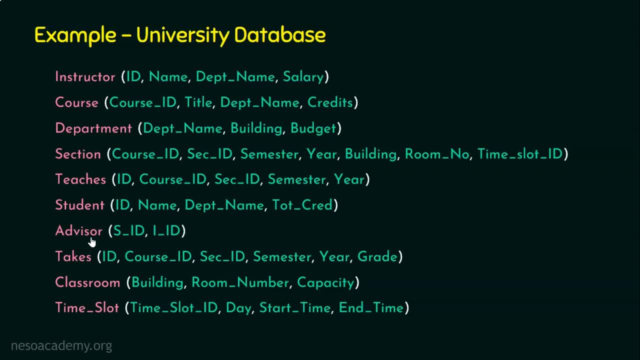 which instructor. So this advisor relation is actually having the relationship between the student ID and the instructor ID. Then takes who takes the course student, right. so the student ID, the course information. Then what about classrooms? every university will have classrooms, right. so classroom related information in the classroom. what are all the information? the building name, the room number. 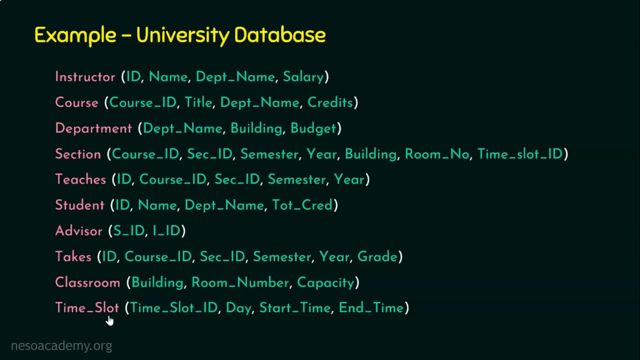 the capacity of the classroom. and what about time slot? Say, for example, for certain courses that university may offer the timing from 9 to 5. for certain other courses it may be from 10 to 6.. So the time slot needs to be maintained. so we need to ensure what is the time slot ID, the day.